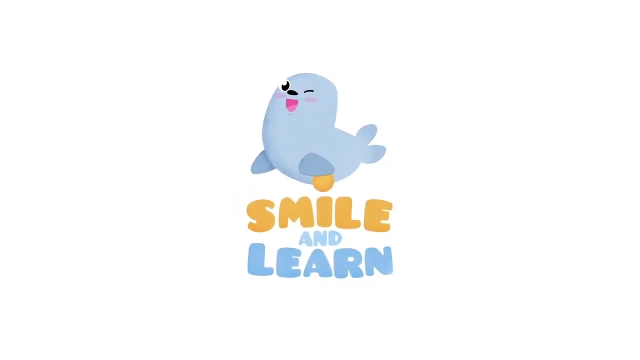 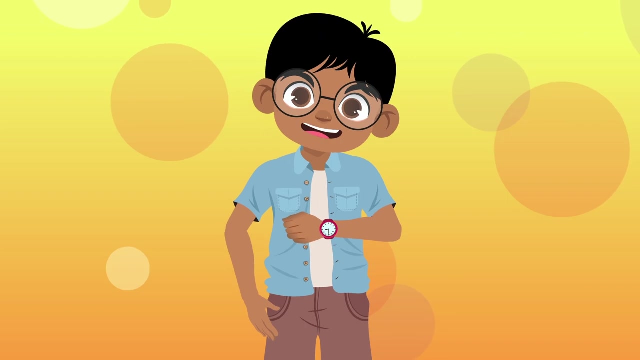 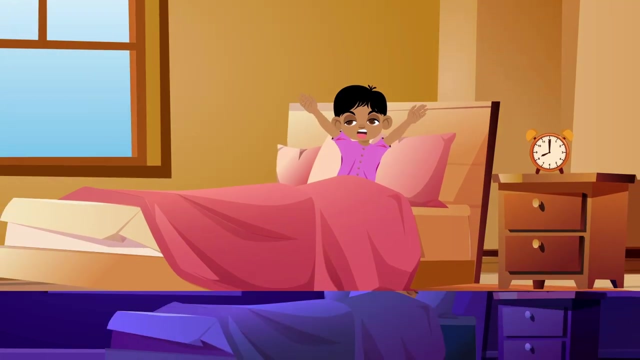 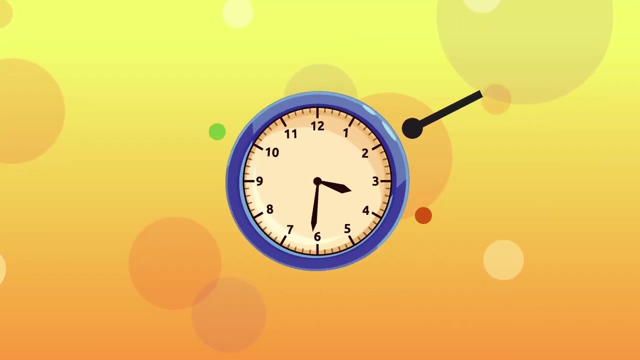 Smile and Learn. Hello everyone, Check out my new watch. It's cool, right. I recently learned how to tell time. It's been great. I know when to wake up or sleep at night so I can have enough rest. Knowing when to do all my activities helps me plan my day at the right time. 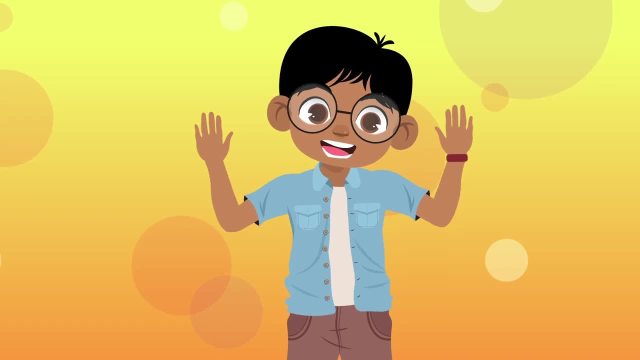 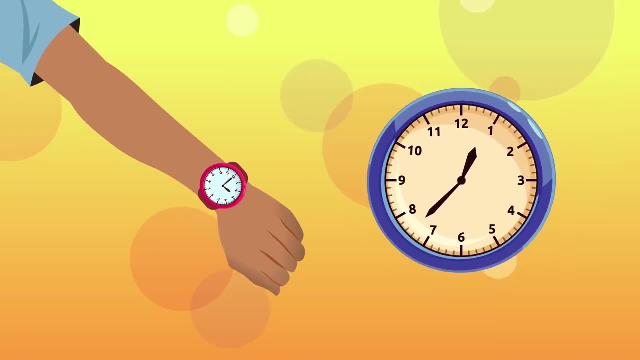 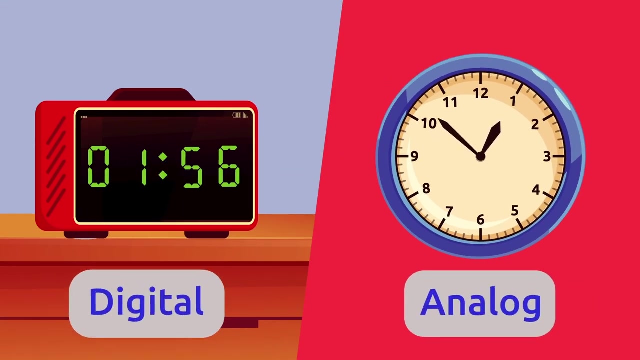 Time. Do you want to see how time works? Let's find out. We tell time using watches or clocks like the ones you see in a classroom. There are two types of clocks: a digital clock and an analog clock. A digital clock tells time with numbers. 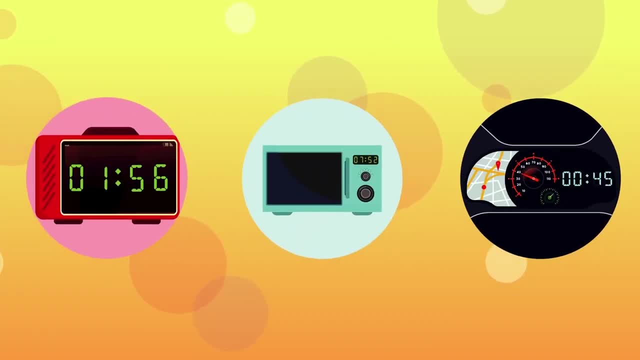 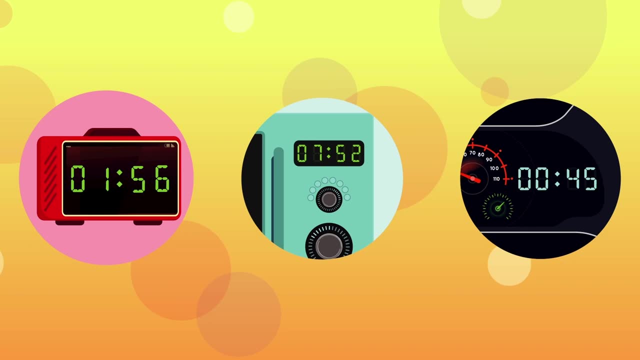 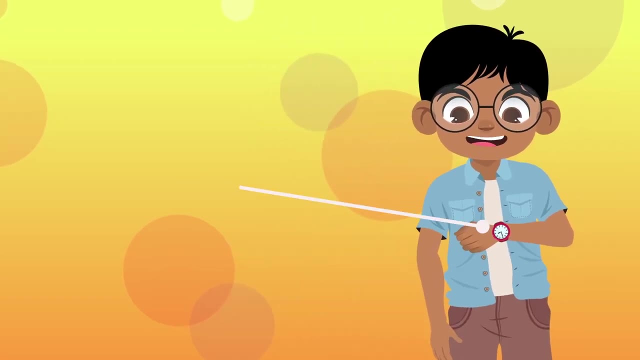 Some examples might be a digital alarm clock, a digital clock on a microwave Or the digital clock in a car. The other type of clock is called an analog clock, which we will look at in more depth today. It's like the one I'm wearing. 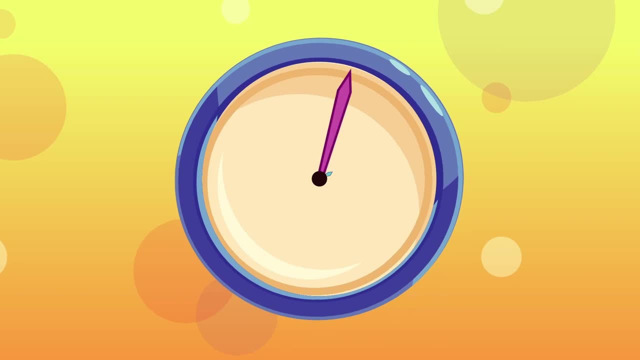 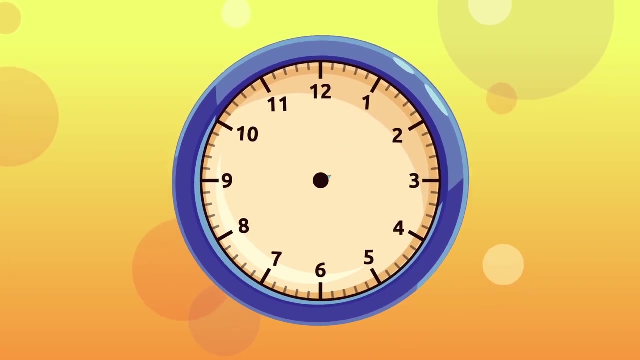 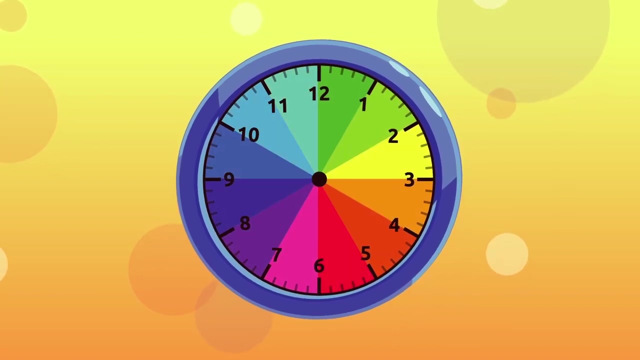 An analog clock shows time with two moving hands that move in a circle on numbers 1 through 12.. Let me show you. It is numbered 1 to 12.. We divide the clock. We divide the clock into 12 sections. Each section equals one hour. 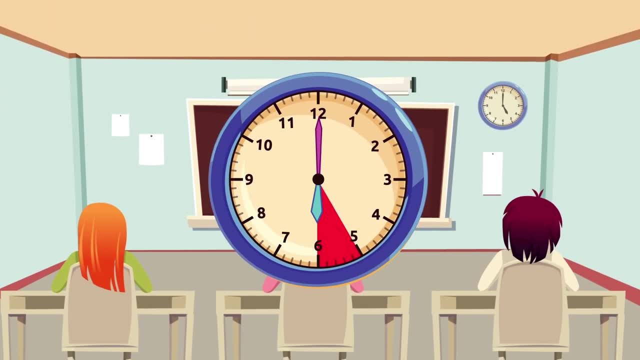 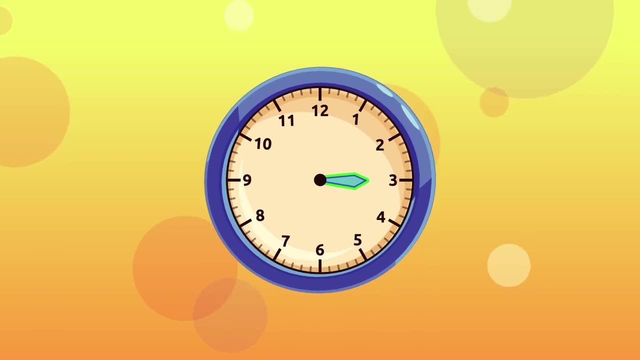 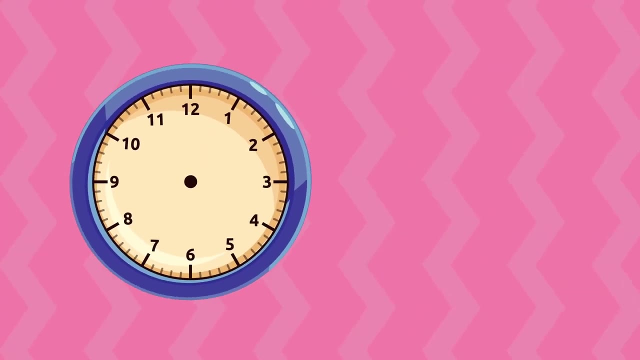 One hour is how long a school period might be. There are also two hands: The shorter one is the hour hand And the longer one is the minute hand. The positions of the hour and the minute hands indicate what part of the day is the hour. 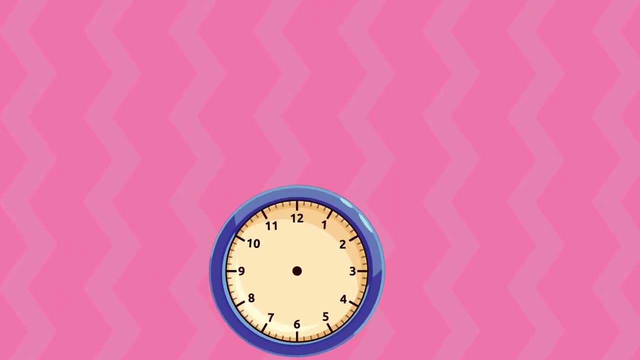 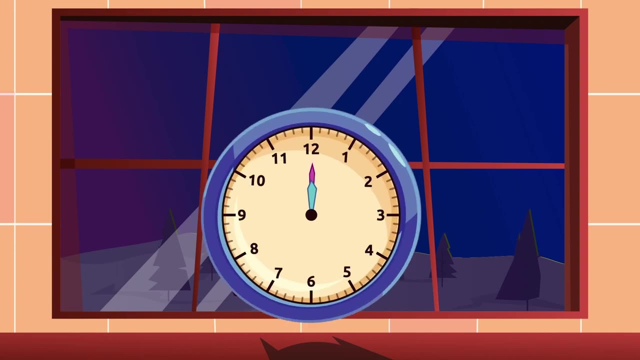 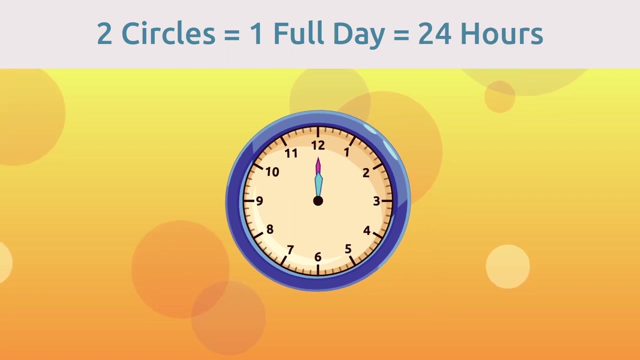 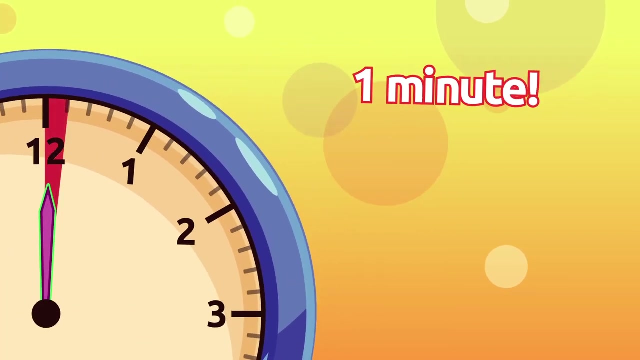 The hour hand moves from one section to another as the day goes by. It takes two circles around the clock to complete a full day, which is 24 hours. The minute hand moves faster than the hour hand. A minute is how long you might take to make chocolate milk. 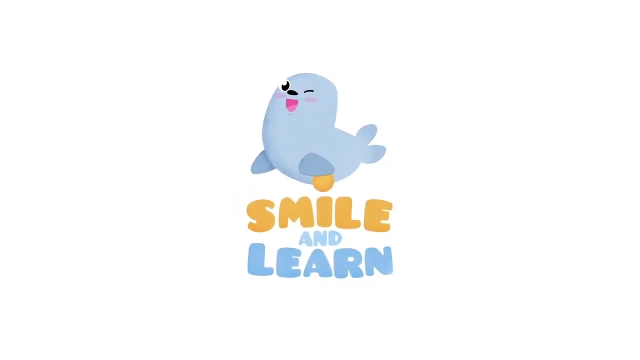 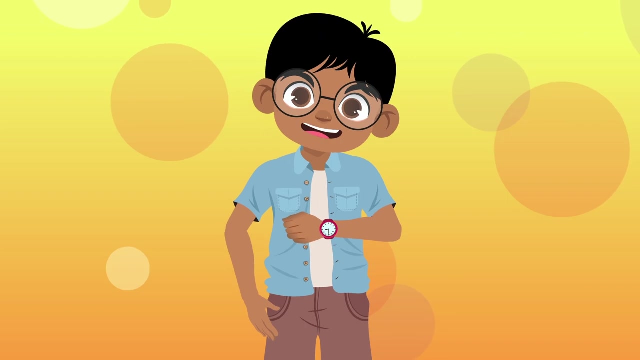 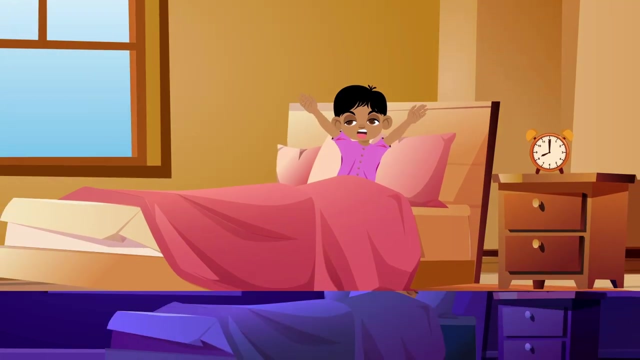 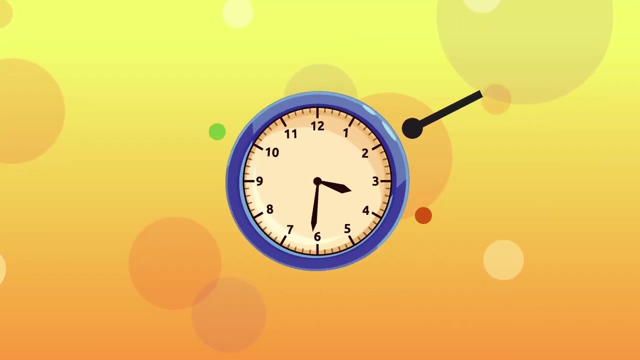 Smile and Learn. Hello everyone, Check out my new watch. It's cool, right. I recently learned how to tell time. It's been great. I know when to wake up or sleep at night so I can have enough rest. Knowing when to do all my activities helps me plan my day at the right time. 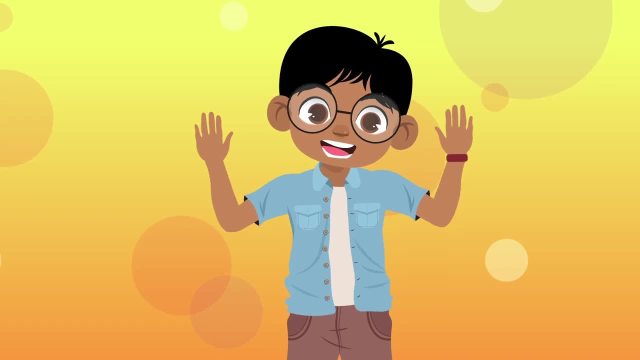 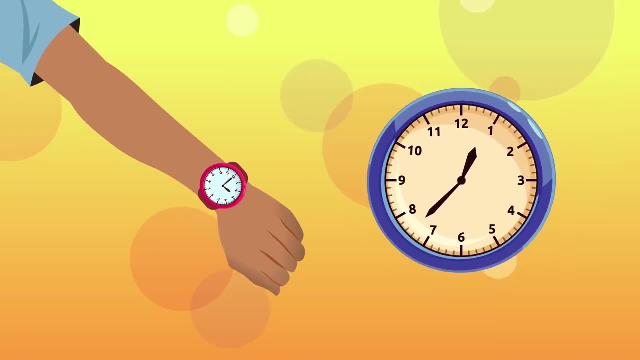 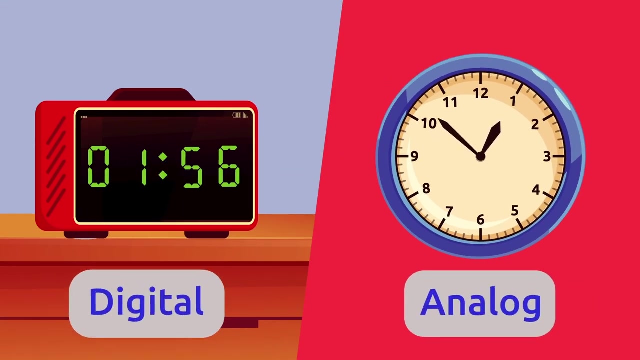 Time. Do you want to see how time works? Let's find out. We tell time using watches or clocks like the ones you see in a classroom. There are two types of clocks: a digital clock and an analog clock. A digital clock tells time with numbers. 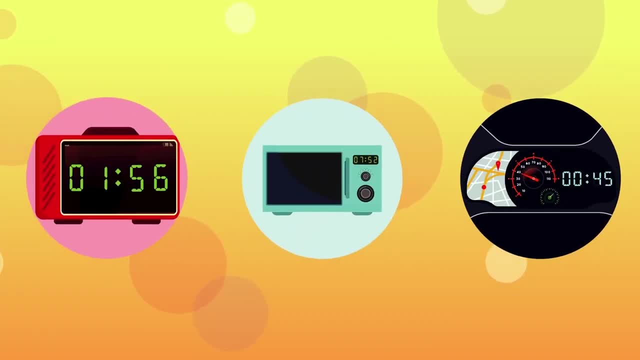 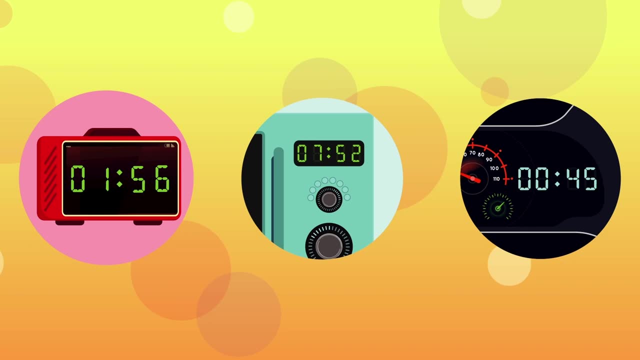 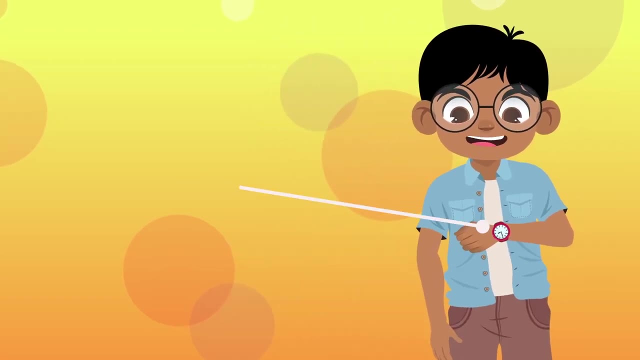 Some examples might be a digital alarm clock, a digital clock on a microwave Or the digital clock in a car. The other type of clock is called an analog clock, which we will look at in more depth today. It's like the one I'm wearing. 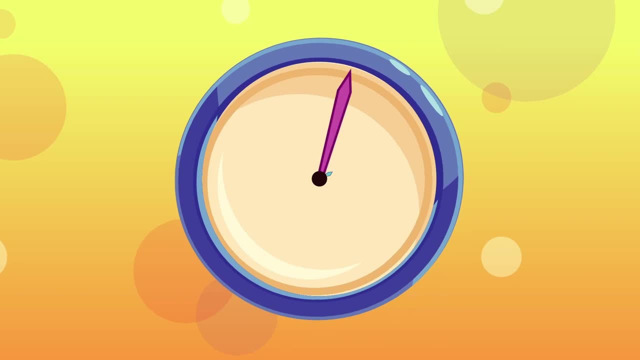 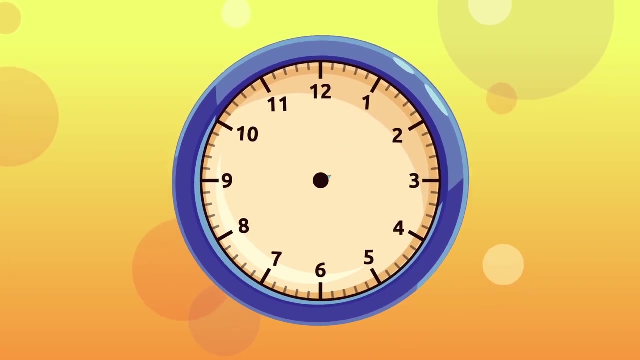 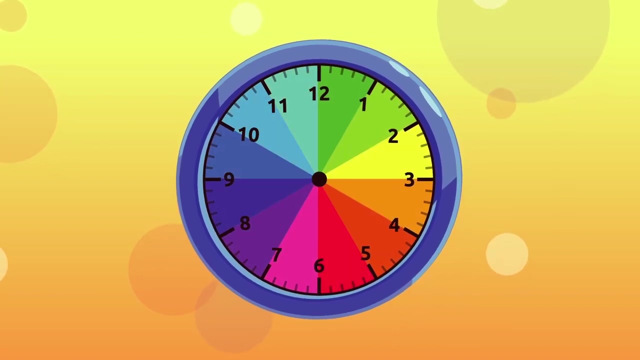 An analog clock shows time with two moving hands that move in a circle on numbers 1 through 12.. Let me show you. It is numbered 1 to 12.. We divide the clock. We divide the clock into 12 sections. Each section equals one hour. 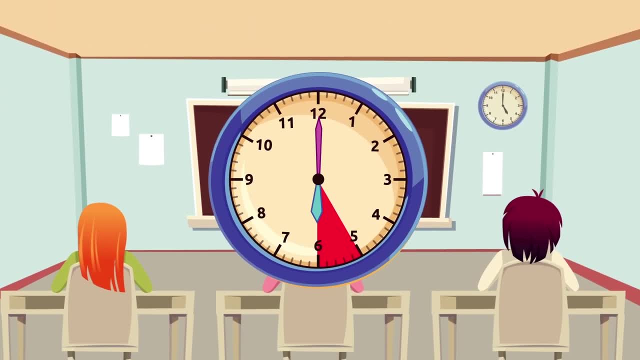 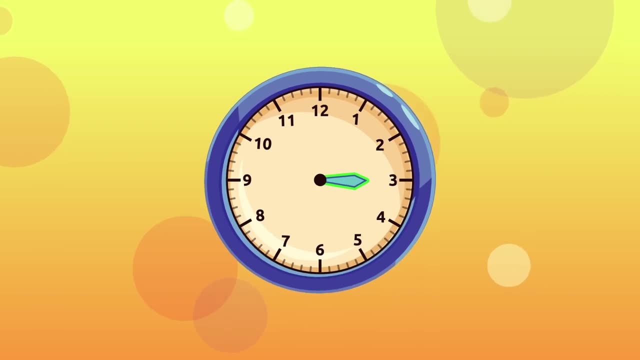 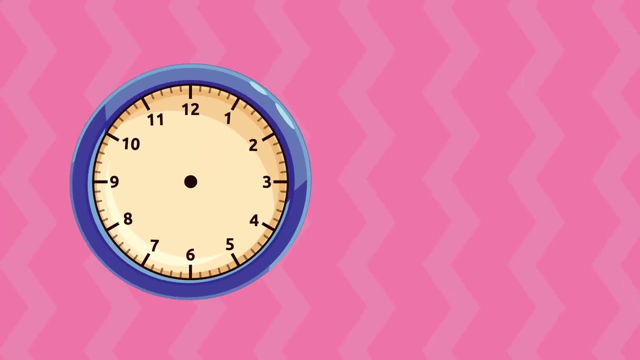 One hour is how long a school period might be. There are also two hands: The shorter one is the hour hand And the longer one is the minute hand. The positions of the hour and the minute hands indicate what part of the day is the hour. 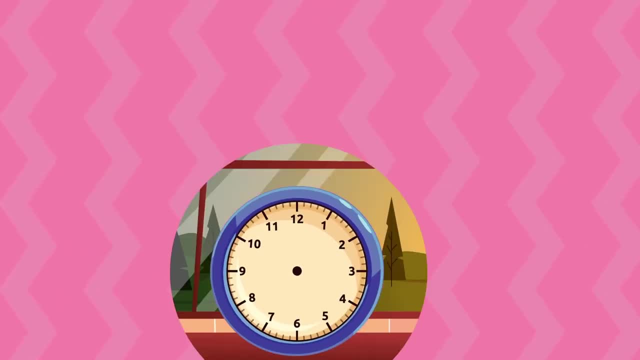 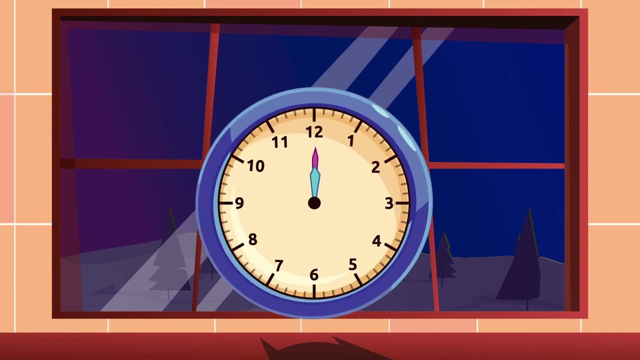 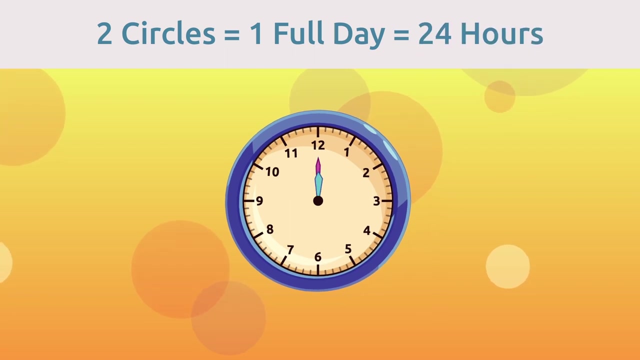 And where does the day we are in? The hour hand moves from one section to another as the day goes by. It takes two circles around the clock to complete the full day, which is 24 hours. The minute hand moves faster than the hour hand. 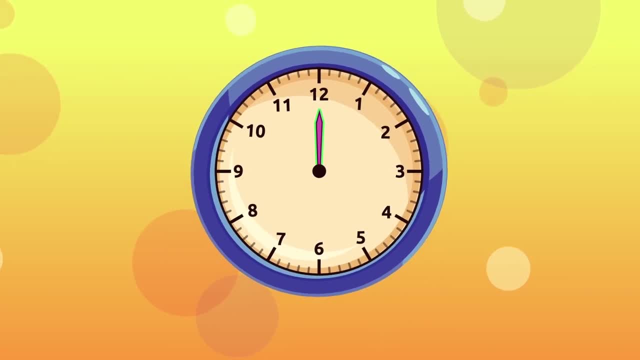 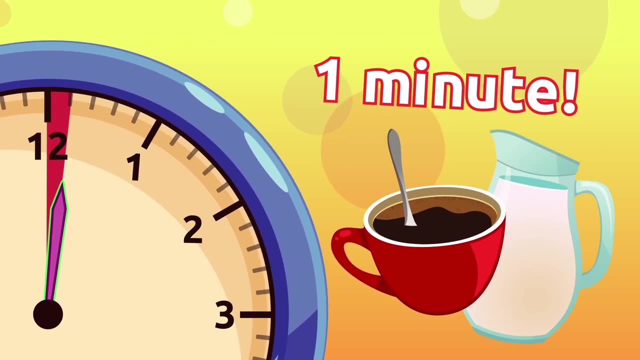 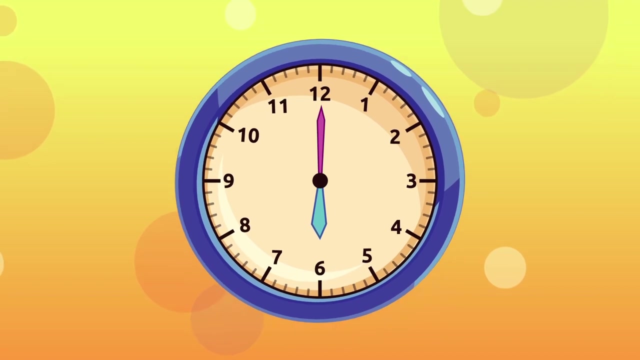 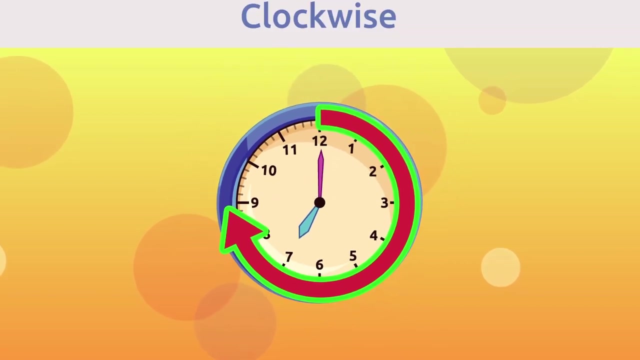 The minute hand moves faster than the hour hand. A minute is how long it might take to make chocolate milk YUM. one circle made by the minute hand around the clock equals one hour. both the hour and minute hands move in the same direction, from 1 to 12 towards the right. this is called clockwise. 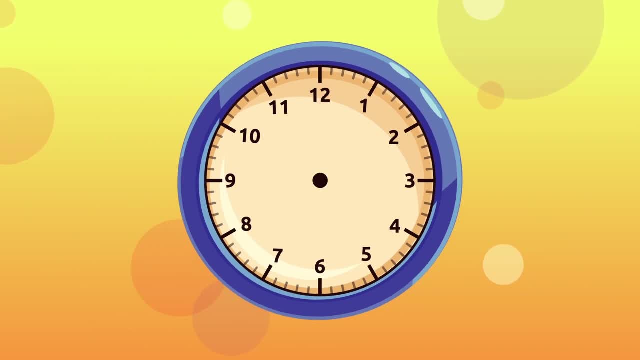 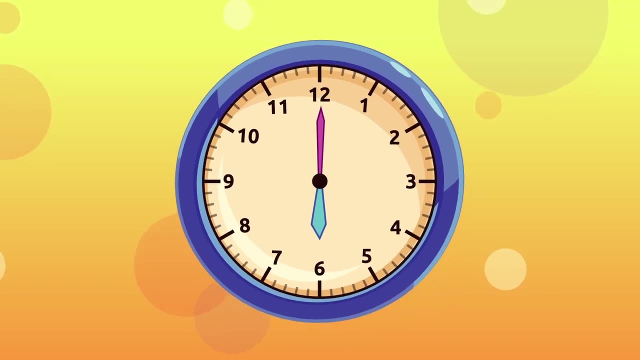 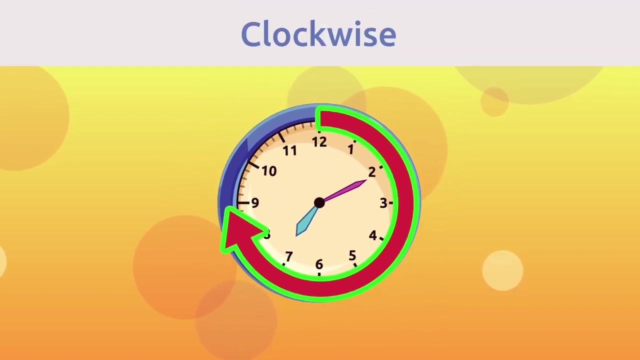 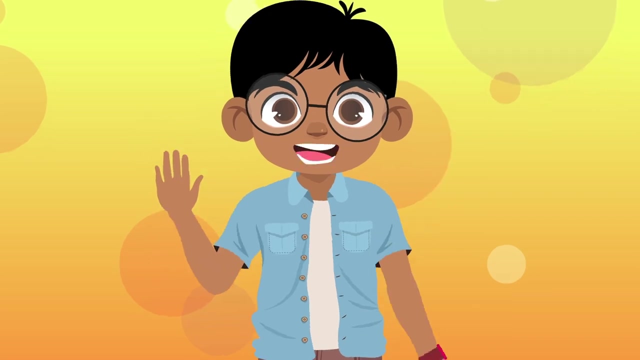 Yum. one circle made by the minute hand around the clock equals one hour. both the hour and minute hands move in the same direction, from 1 to 12 towards the right. this is called clockwise blocks. can be fascinating, right? wow, it's my lunch time. i'm hungry. check out the following videos. 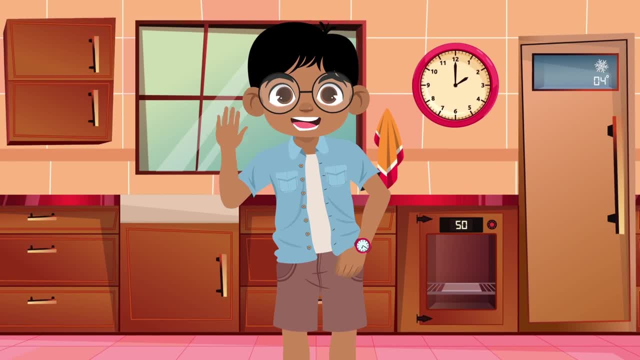 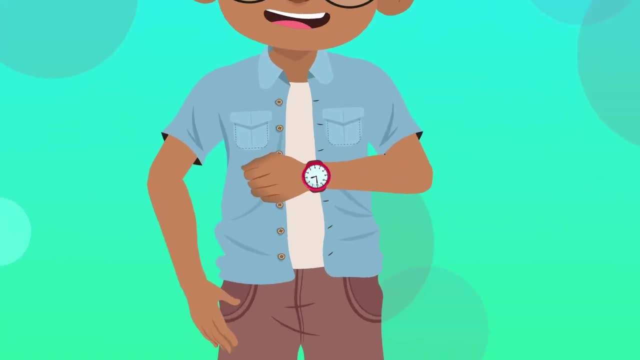 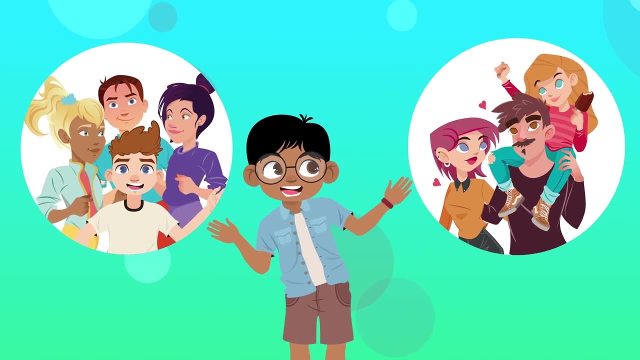 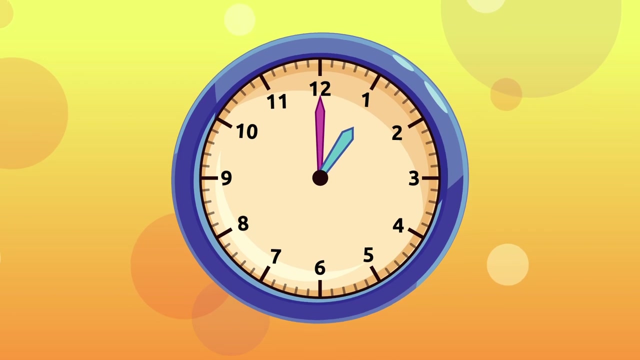 where we will learn about how to tell time. see you soon. hey, everyone, i love my new watch. i've been practicing how to tell time to know how i'll be spending my day with friends and family. first we'll learn how to say the hours when the minute hand is on the number 12 and the hour hand. 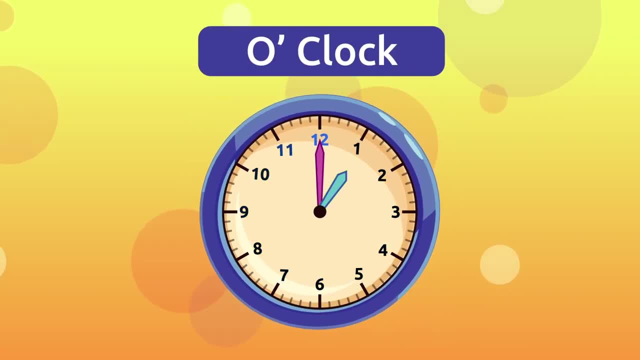 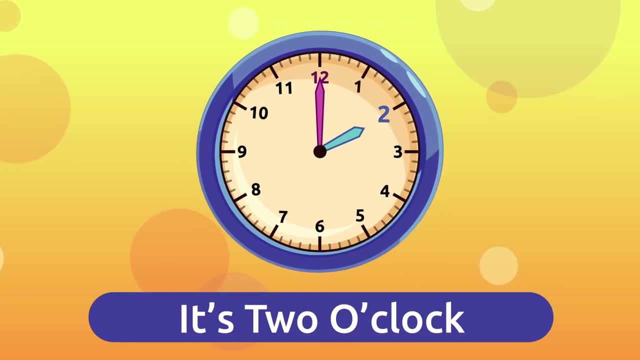 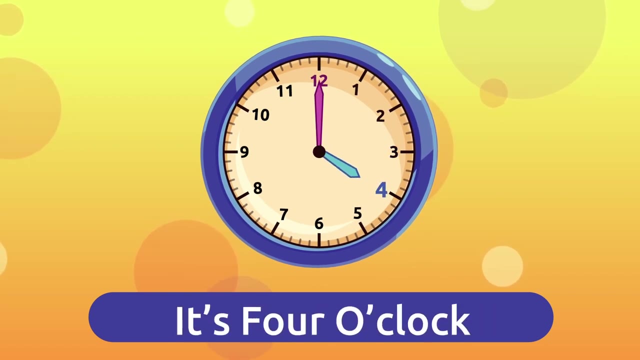 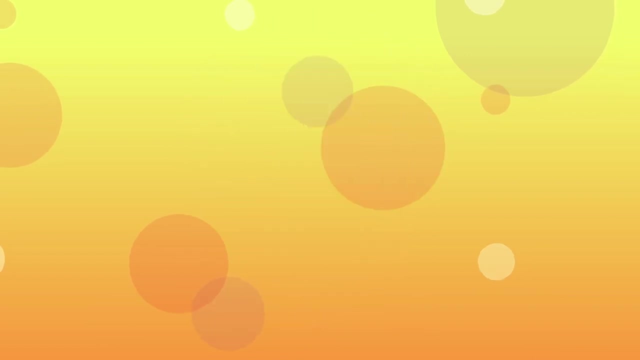 is on any number. we say that number and a clock. for example, it's one o'clock, it's two o'clock, it's three o'clock, it's four o'clock and it's five o'clock. see how easy it is. now you try. could you tell me what time it is? 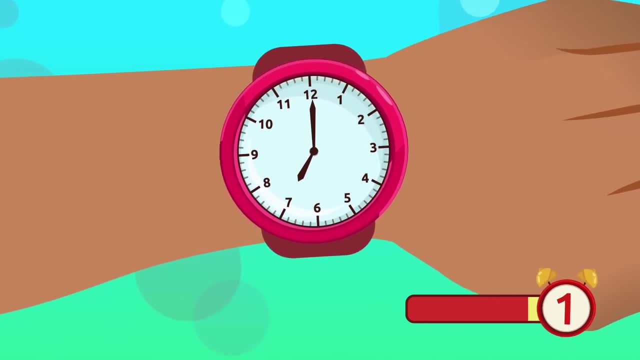 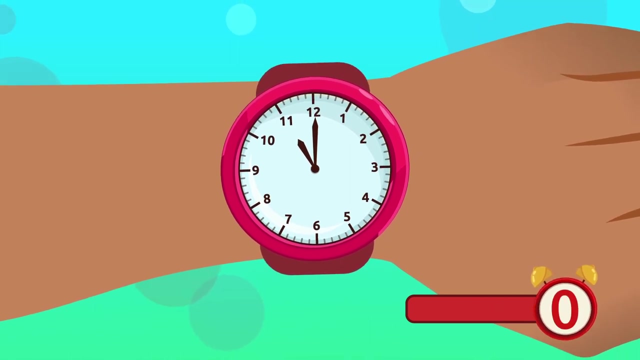 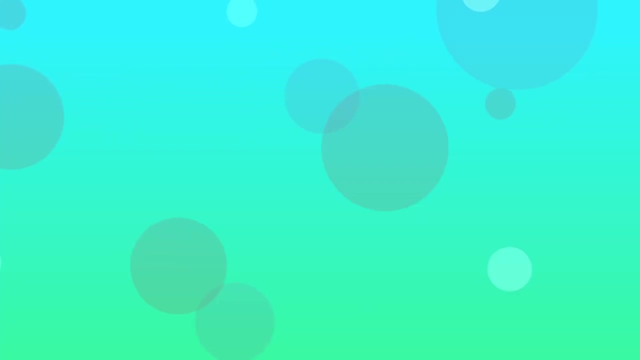 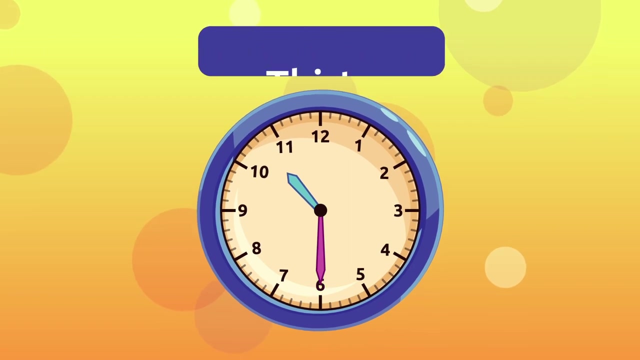 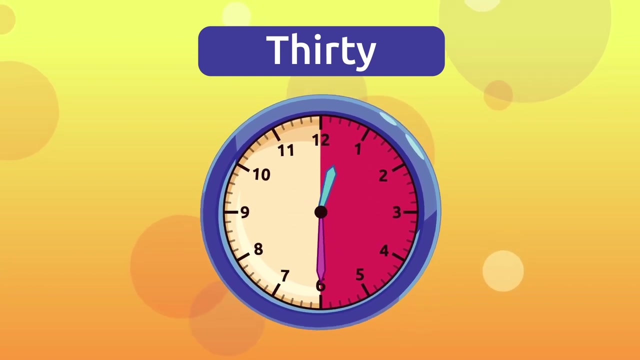 it's seven o'clock- awesome. what time is it? it's eleven o'clock- awesome. what happens when the minute hand is on the number six? say the hour first and then add 30.. Since the clock is divided into 12 parts, when the minute hand is in the middle, that is, on the number 6, and the hour hand is on one of the numbers. 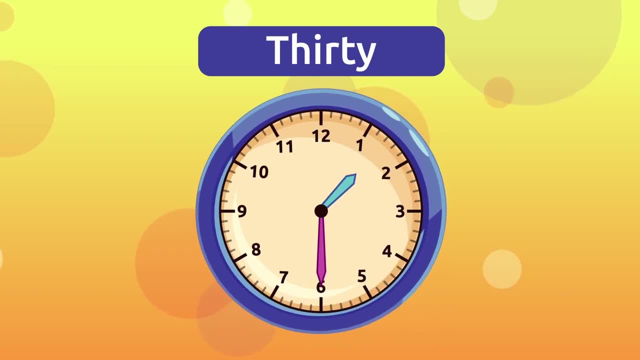 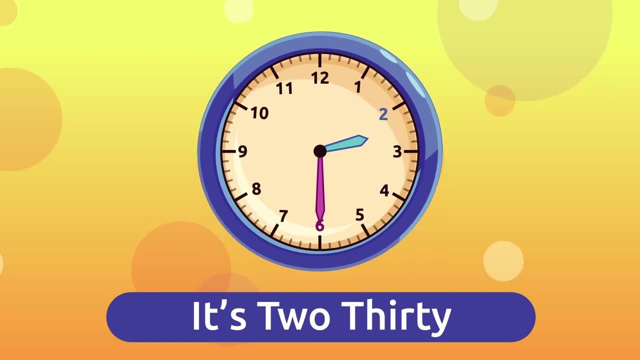 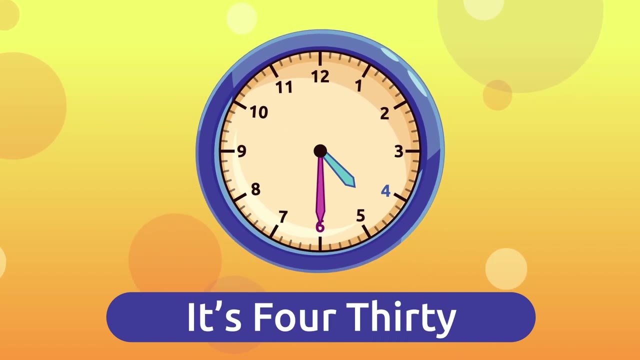 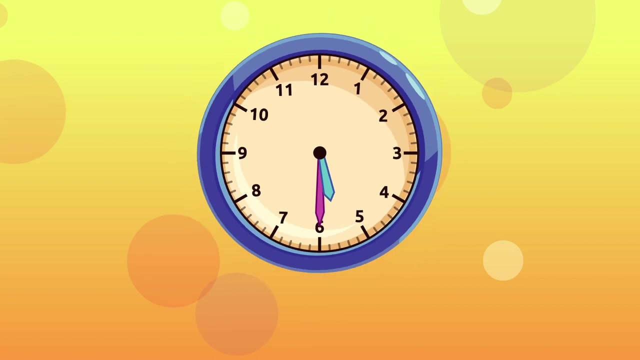 we say: it is that hour and 30.. For example, it's 1.30.. It's 2.30.. It's 3.30.. It's 4.30.. And it's 5.30.. Now it's your turn. What time is it? 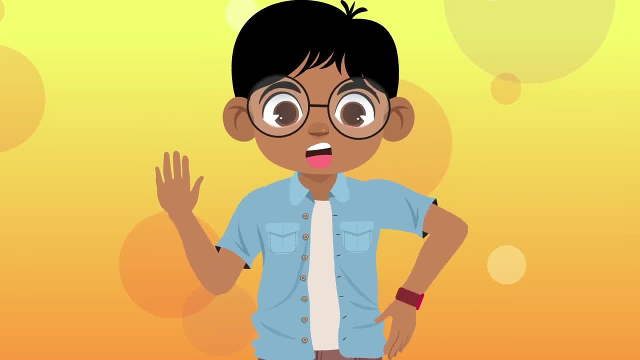 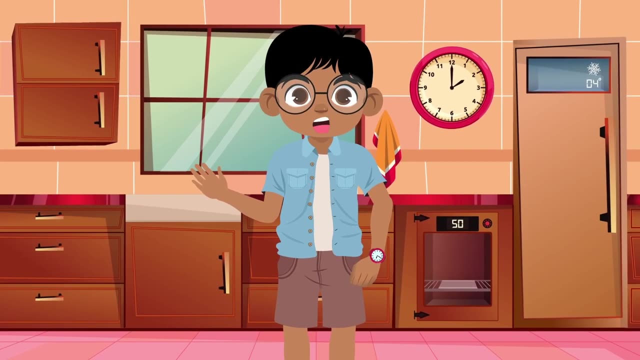 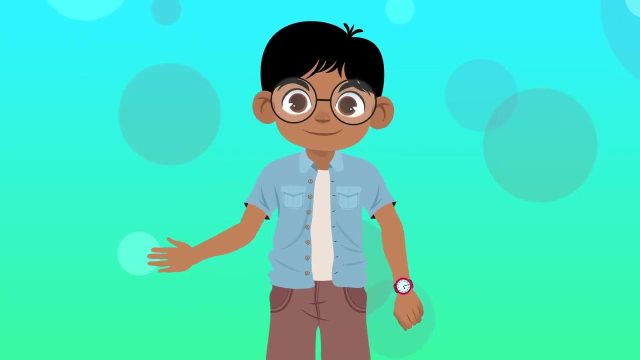 blocks can be fascinating, right? wow, it's my lunch time. i'm hungry. check out the following videos where we will learn about how to tell time. see you soon. hey, everyone, i love my new watch. i've been practicing how to tell time to know how i'll be spending my day with friends and family. 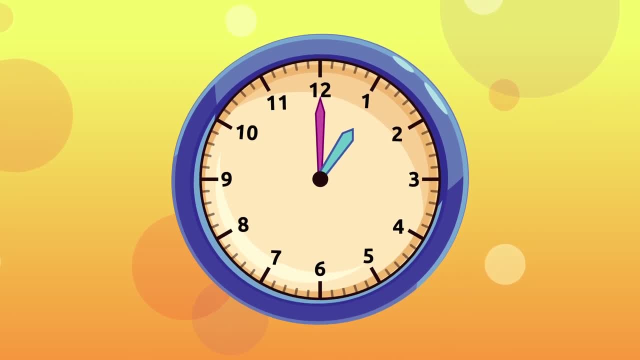 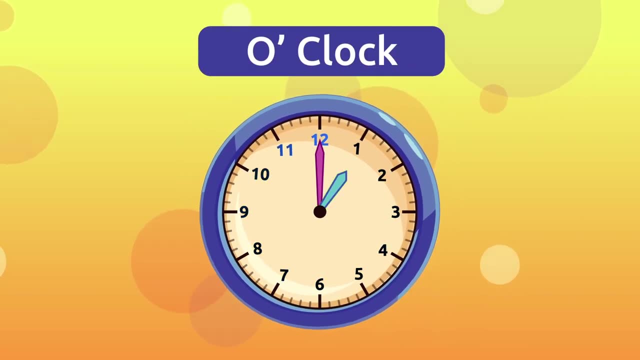 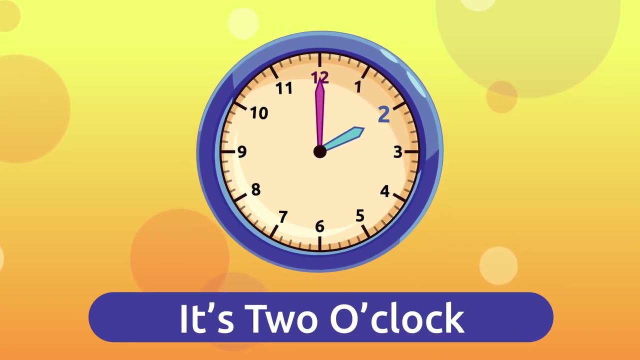 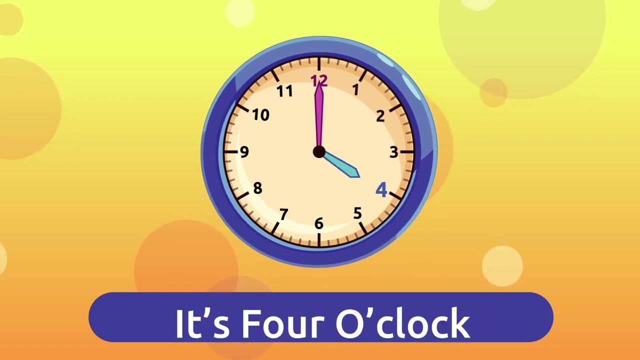 first we'll learn how to say the hours. when the minute hand is on the number 12 and the hour hand is on any number, we say that number and a clock. for example: it's one o'clock, it's two o'clock, it's three o'clock, it's four o'clock. 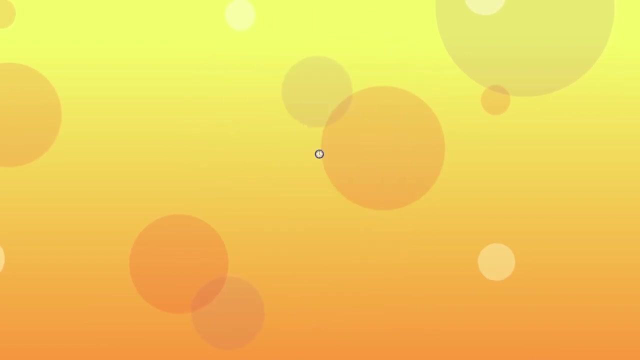 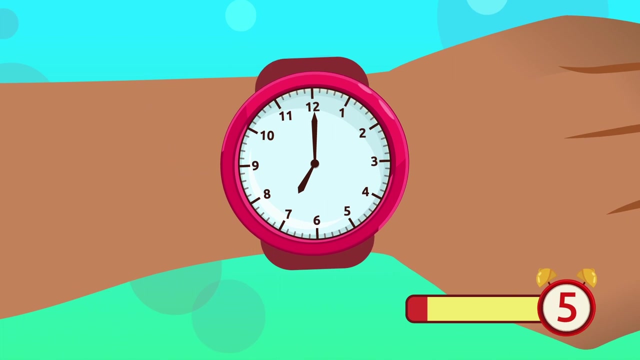 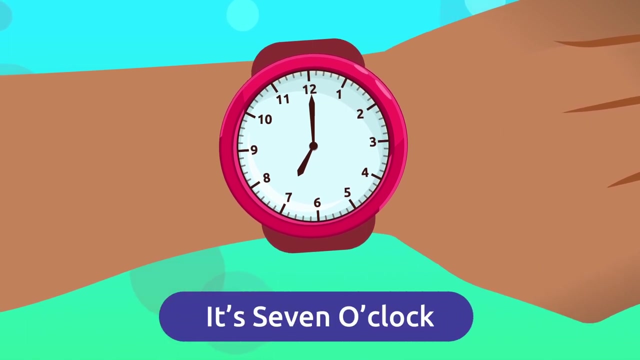 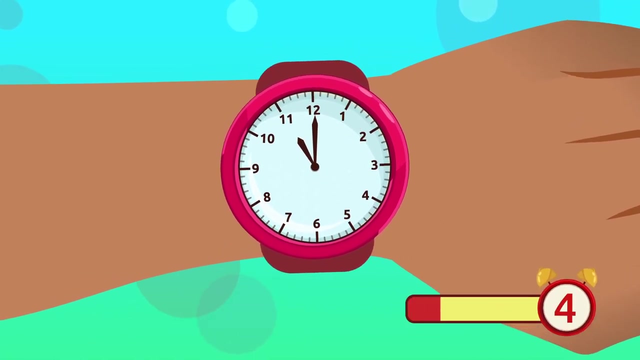 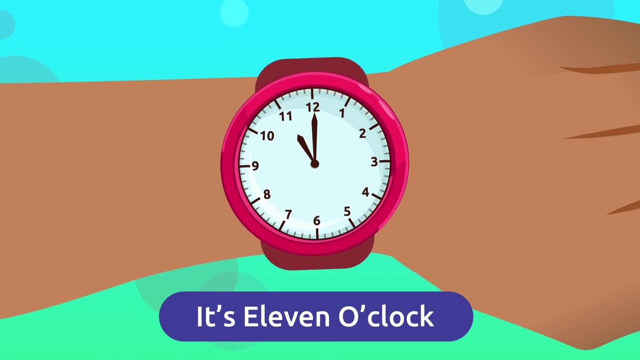 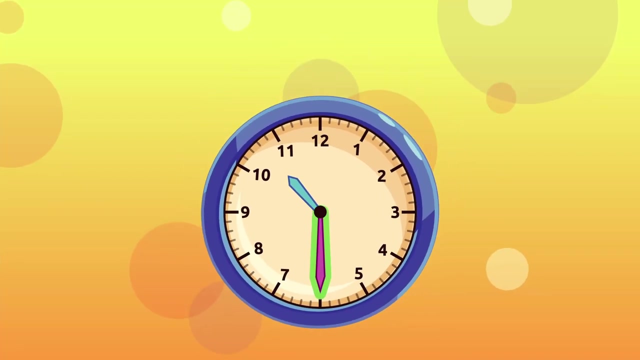 and it's five o'clock see how easy it is now you try could you tell me what time it is � it's seven o'clock what time is it it's 11 o'clock awesome what happens when the minute hand is on the number six cheesecake 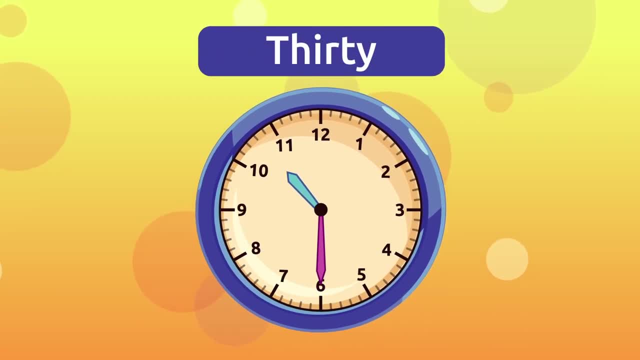 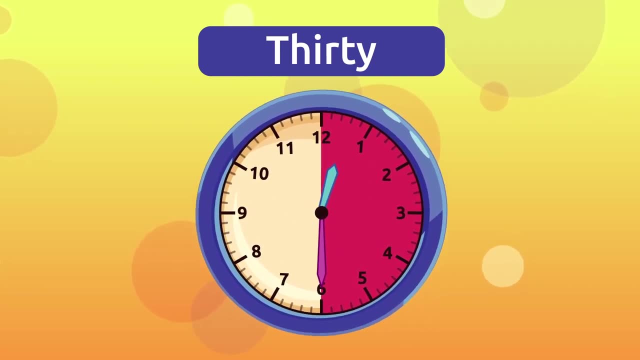 hour first and then add 30. Since the clock is divided into 12 parts, when the minute hand is in the middle, that is on the number 6, and the hour hand is on one of the numbers we say it is. 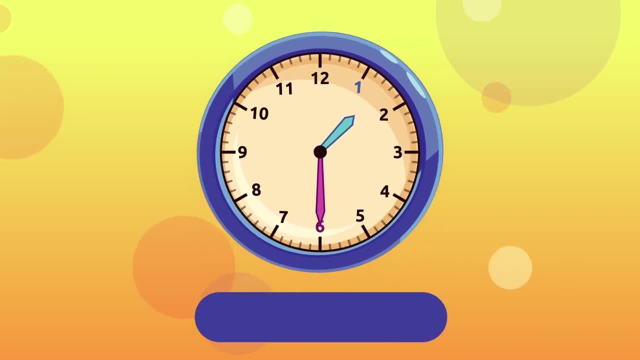 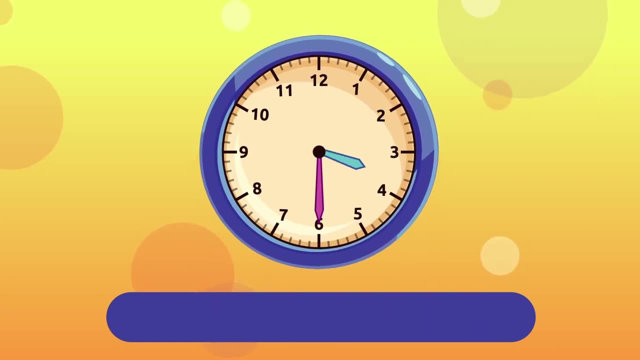 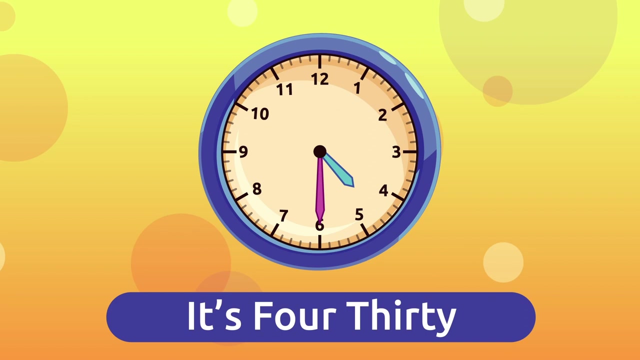 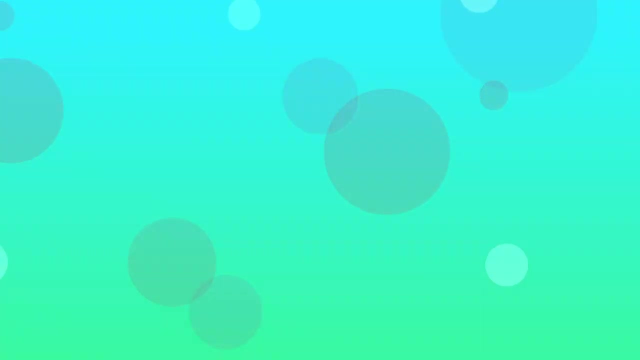 that hour and 30.. For example, it's 1.30.. It's 2.30., It's 3.30.. It's 4.30. And it's 5.30.. Now it's your turn. What time is it? 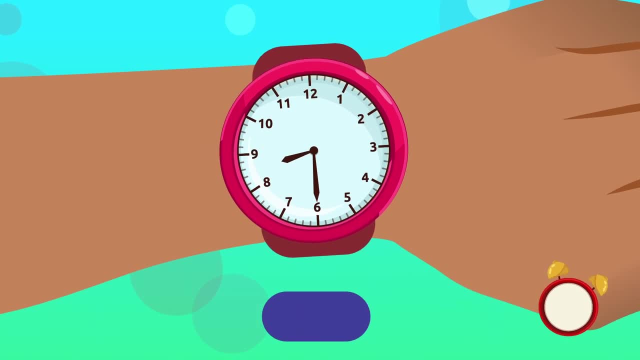 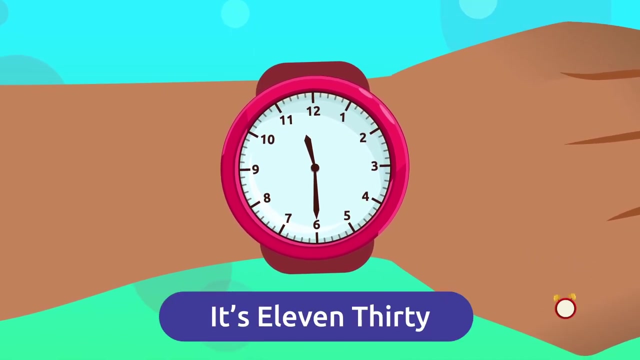 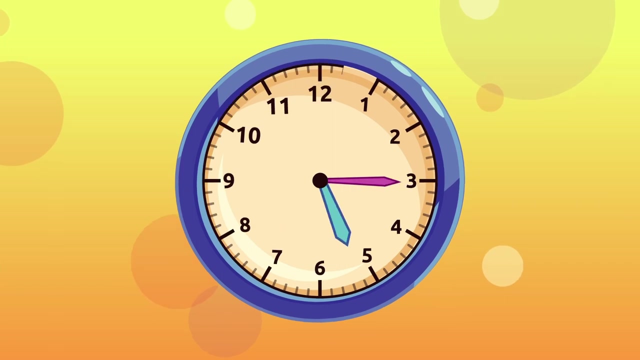 That's right, It's 8.30.. And now, what time is it? That's it, It's 11.30.. When the minute hand is on the 3,, in other words, a quarter of an hour has passed, We say that it is. 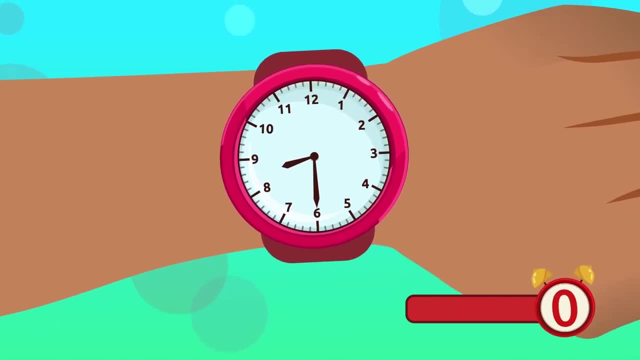 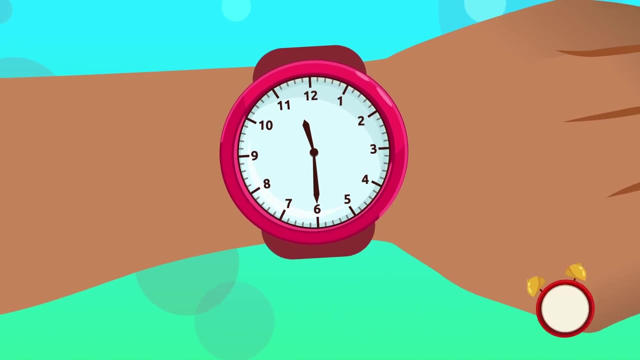 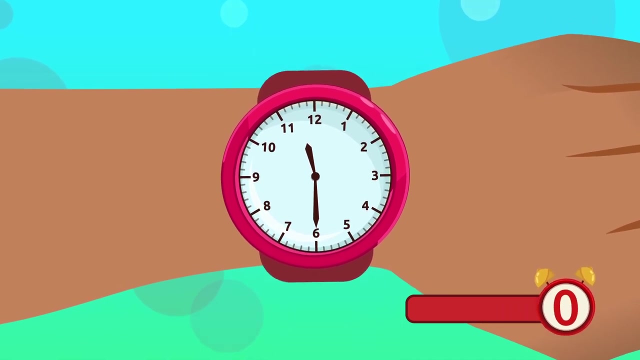 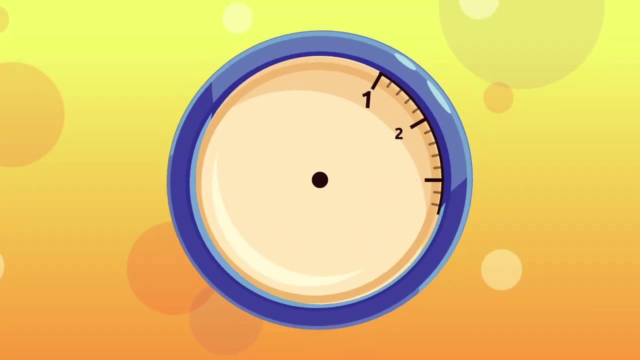 8.30.. That's right, It's 8.30.. And now, what time is it? That's it, It's 11.30.. When the minute hand is on the 3,, in other words, a quarter of an hour has. passed. We say that it is 8.30.. And now what time is it? It's 11.30.. When the minute hand is on the 3,, in other words, a quarter of an hour has passed, We say that it is a quarter after the. 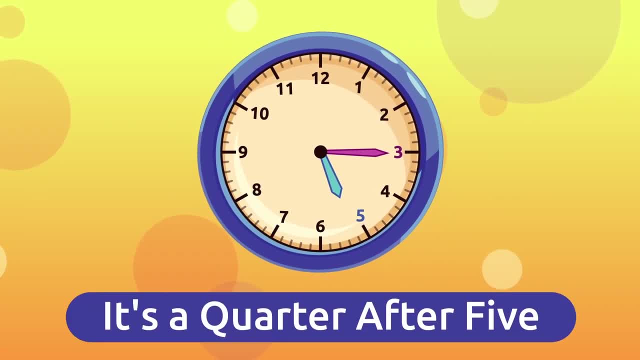 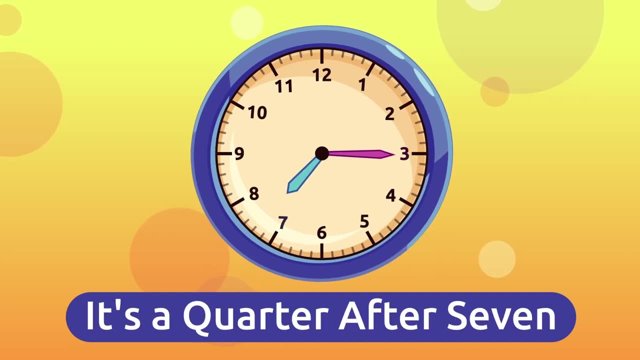 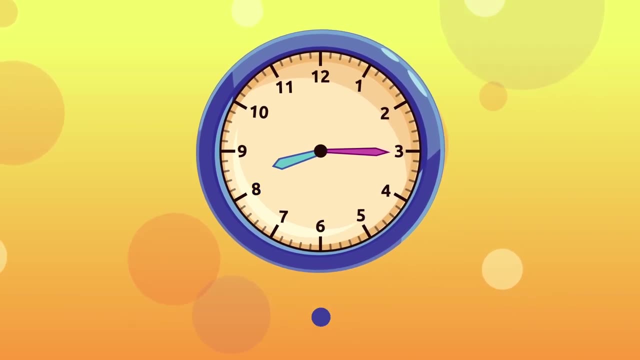 hour, For example, it's a quarter after 5.. It's a quarter after 6.. It's a quarter after 7. And it's a quarter after 8.. How about you give it a try? What time is it? 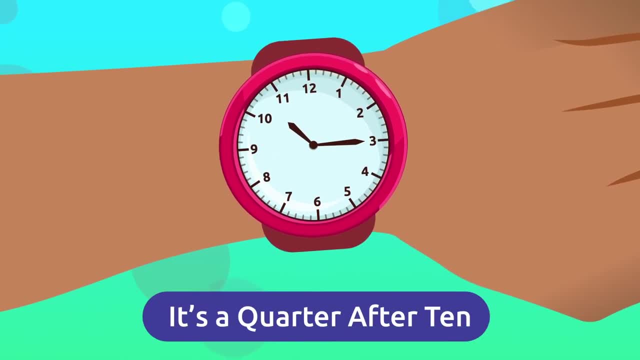 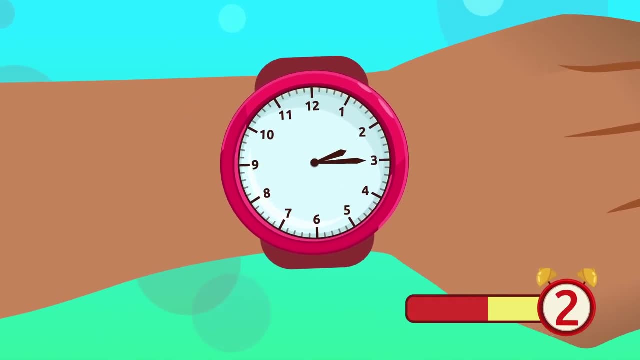 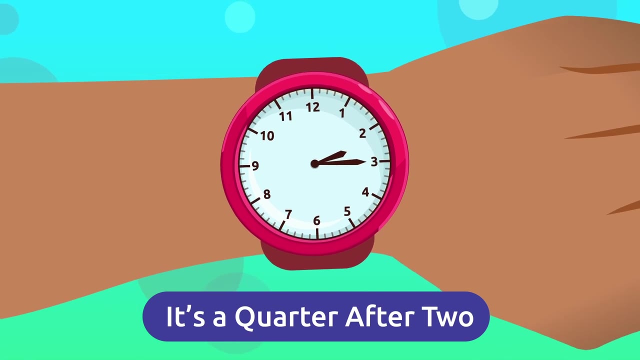 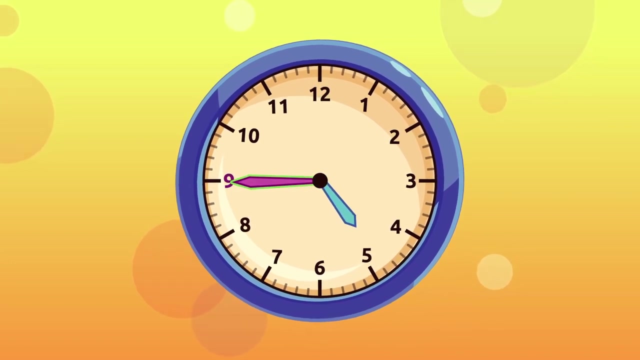 It's a quarter after 10.. Very good, How about now? What time is it? It's a quarter after 2.. Good job. Finally, let's see what happens if we move the minute hand to the number 9.. How would you say? this time, As you can see, it is moved from 1 to 9.. 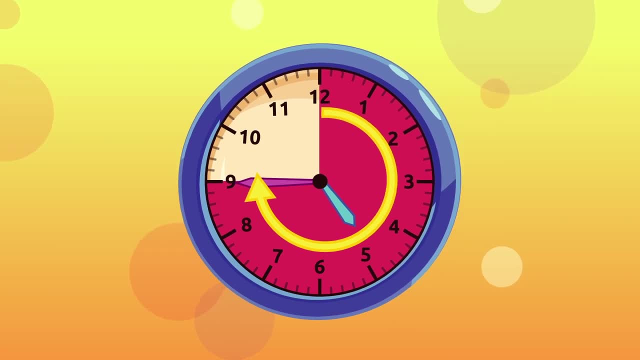 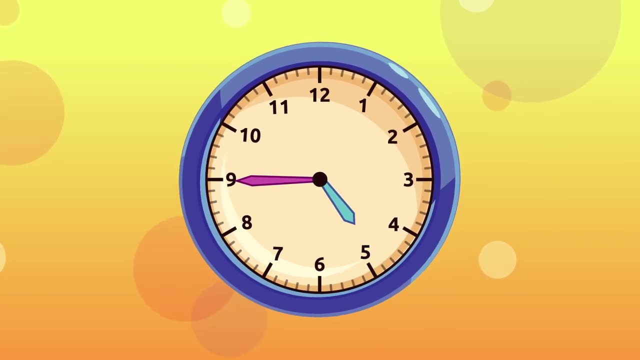 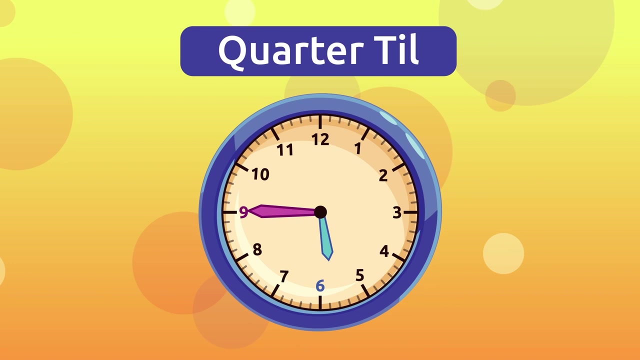 It is moved from the number 12 to the number 9.. There is only a quarter left until it completes the hour. What if the minute hand is on the number 9?? Look at this example: The hour hand is closer to the 6, and the minute hand is on the 9.. That means it's a quarter of an hour left until 6.. 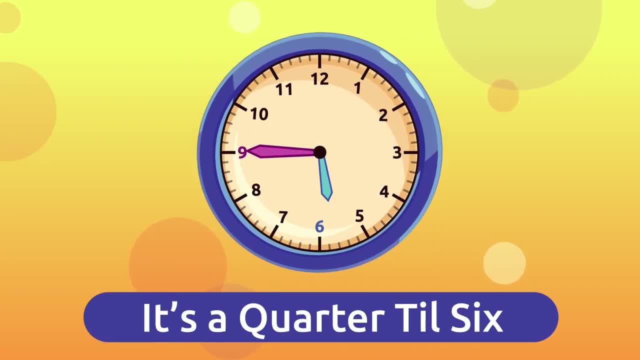 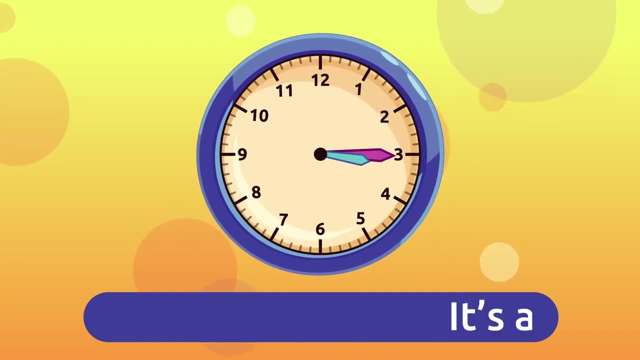 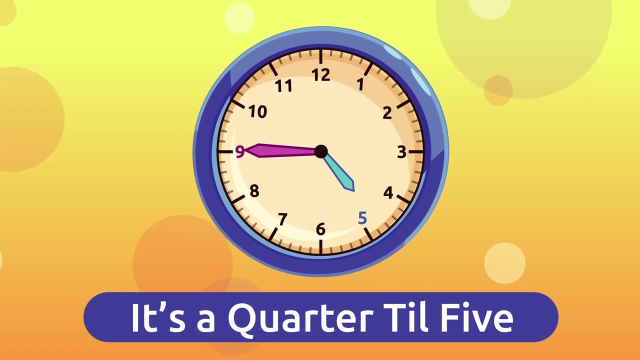 So we say that it is a quarter till 6.. Easy right, It's a quarter till 3.. It's a quarter till 4.. It's a quarter till 5.. All right, now it's your turn. What time is it? 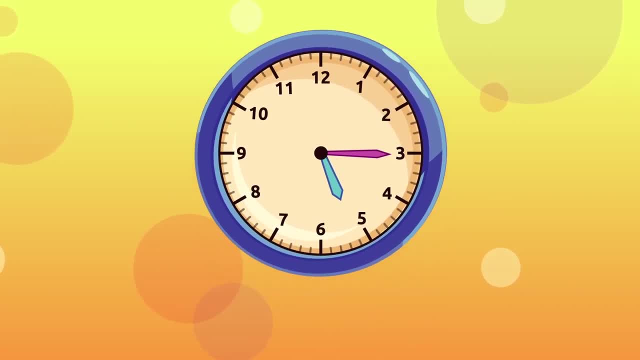 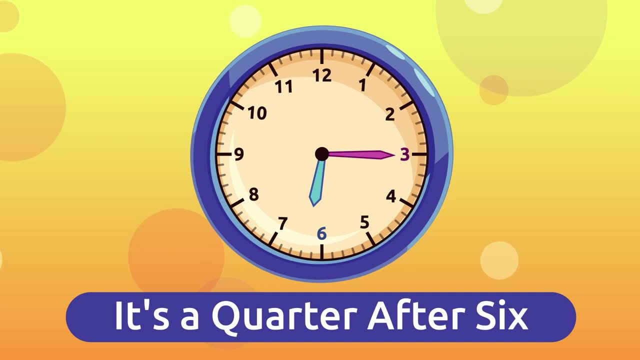 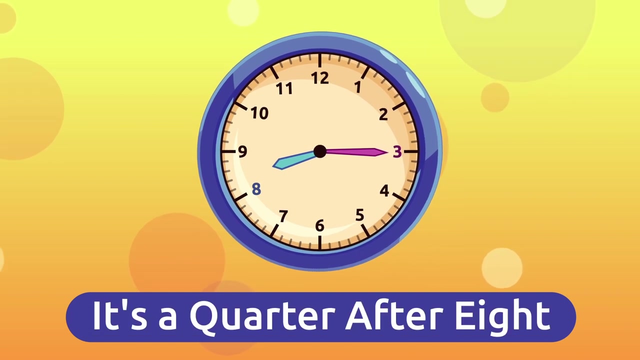 a quarter after the hour, For example. it's a quarter after 5.. It's a quarter after 6.. It's a quarter after 7. And it's a quarter after 8.. How about you give it a try? What time is it? 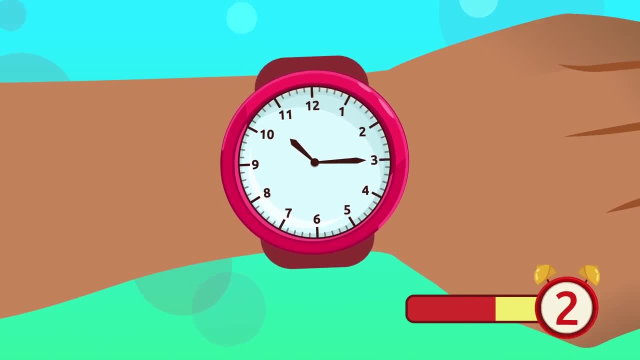 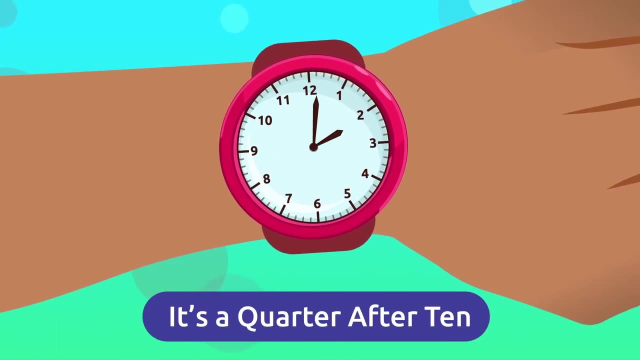 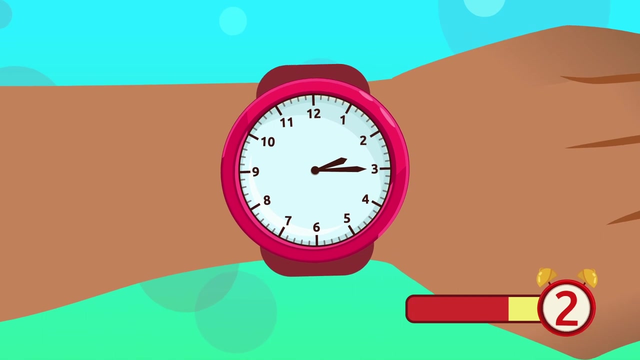 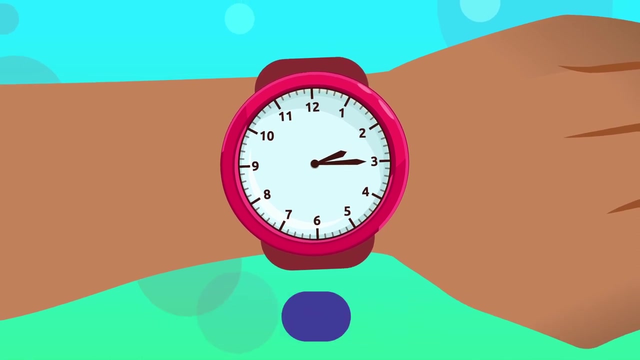 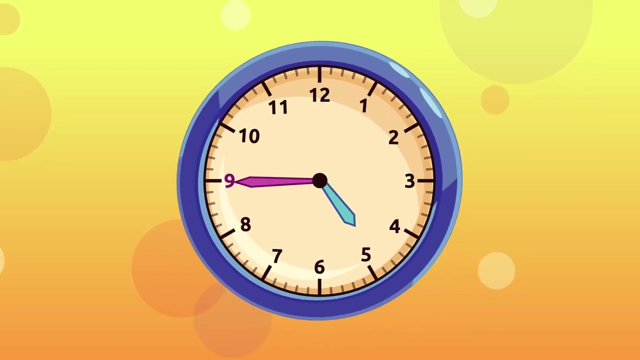 It's a quarter after 10.. Very good, How about now? What time is it? It's a quarter after 2.. Good job. Finally, let's see what happens if we move the minute hand to the number 9.. How would you say this time? 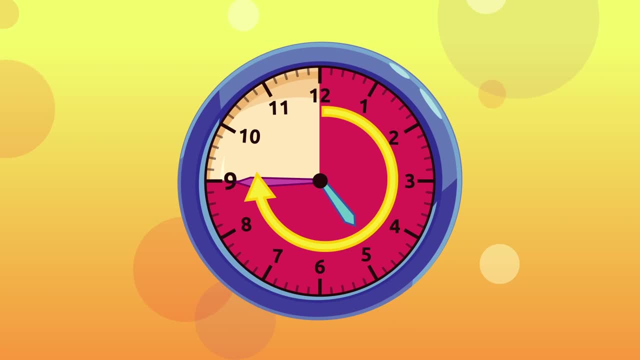 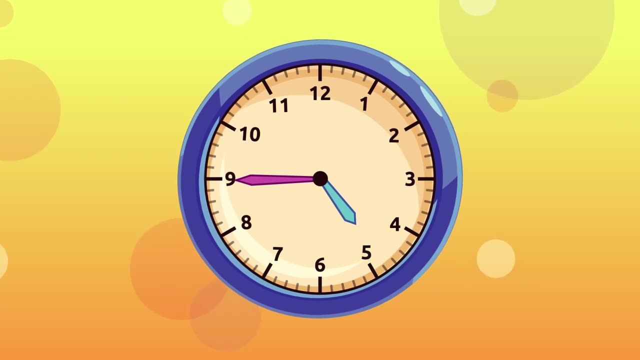 As you can see, it has moved from the number 12 to the number 9.. There is only a quarter left until it completes the hour. What if the minute hand is on the number 9?? Look at this example: The hour hand is closer to the 6 and the minute hand is on the 9.. 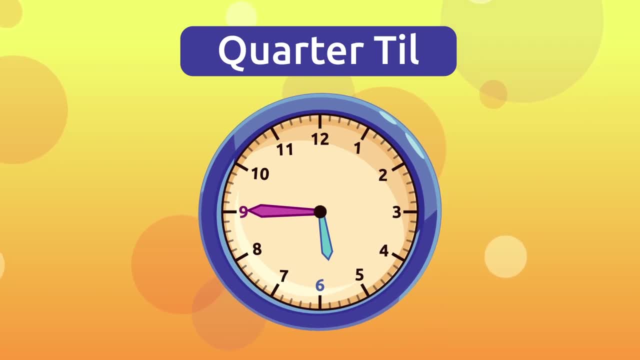 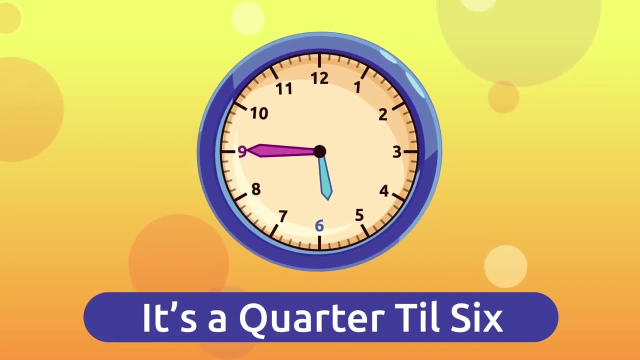 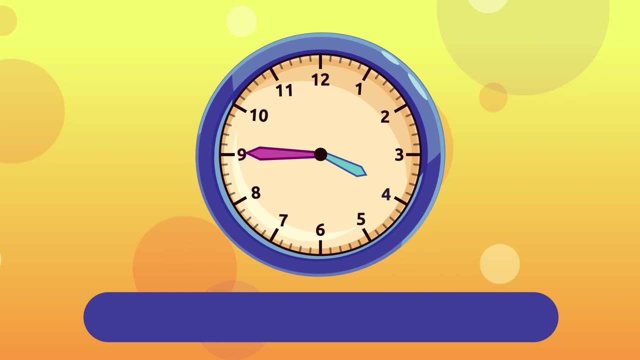 That means it's a quarter of an hour left until 6.. So we say this is a quarter after 22.. So we say that it's a quarter in our hands. say that it is a quarter till six, Easy right, It's a quarter till three, It's a quarter. 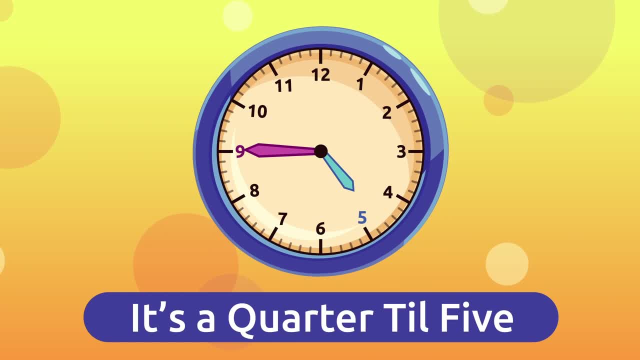 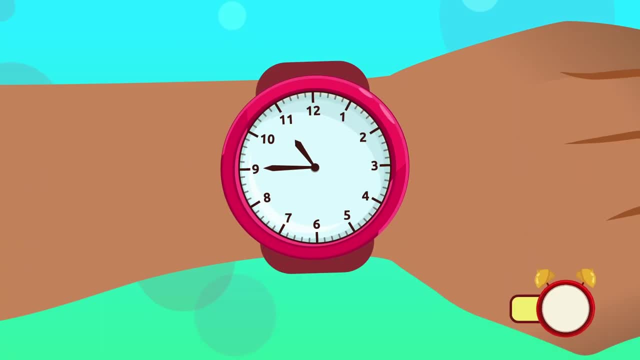 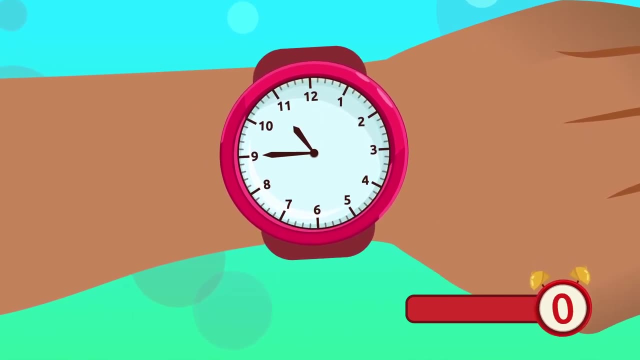 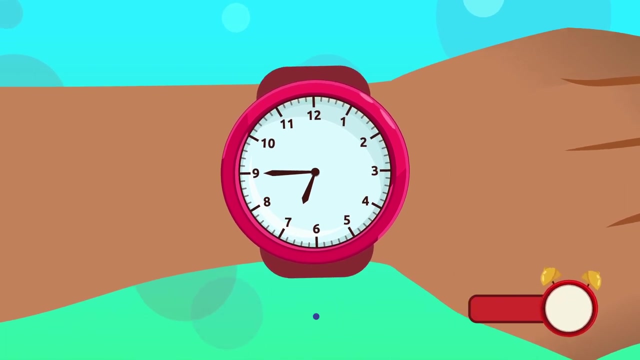 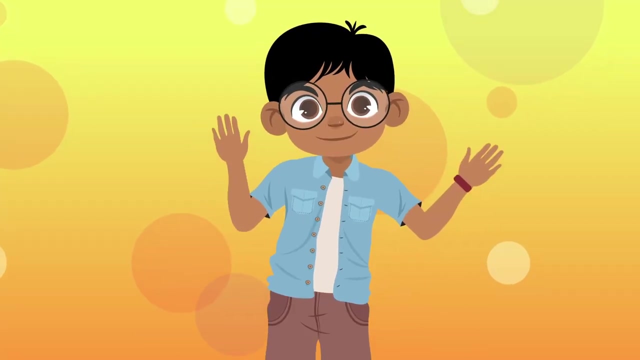 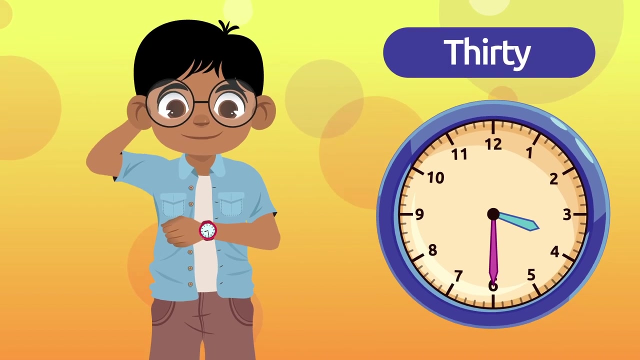 till four. It's a quarter till five. All right, now it's your turn. What time is it? It's a quarter till eleven. Awesome, What time is it? It's a quarter till seven. Super, You did great. You know how to tell time by the hour and by using thirty A quarter.